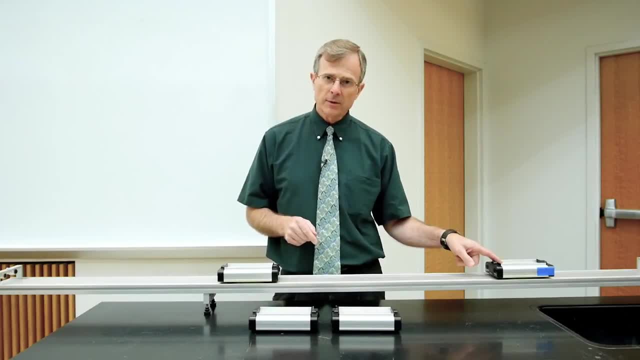 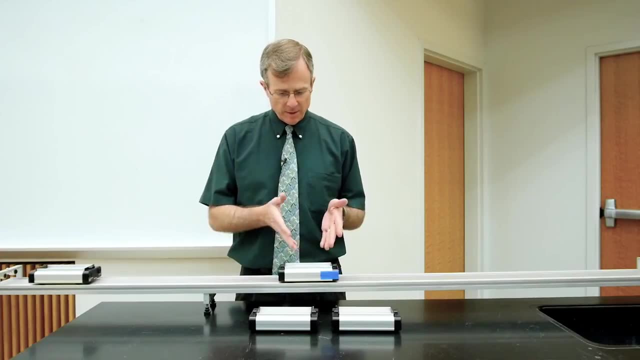 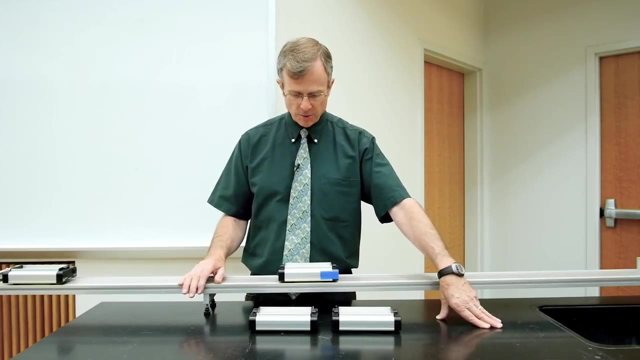 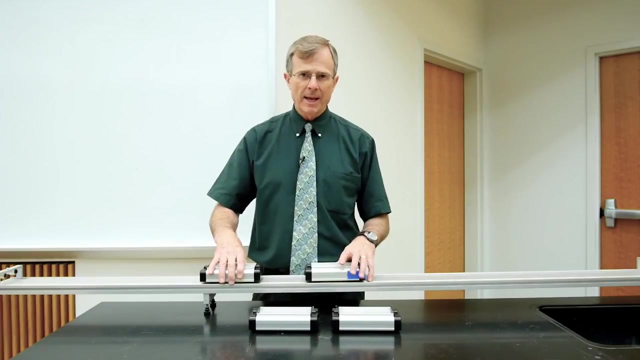 and transferred all of its energy to the other cart, And we can do the same thing in reverse: It transfers all of its energy to the other one. That's a so-called elastic collision, where there's no energy lost in the collision. During the collision, both energy and momentum are conserved. 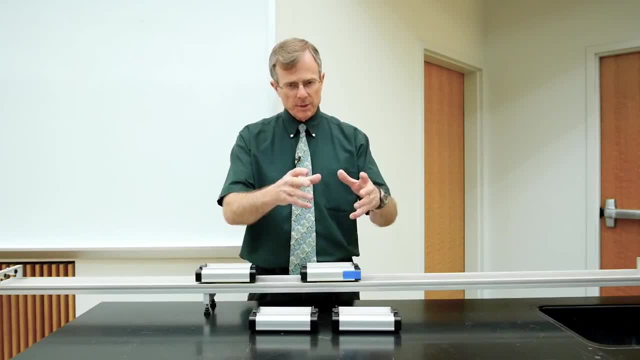 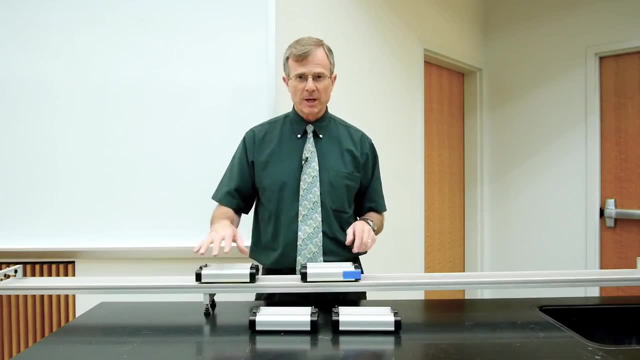 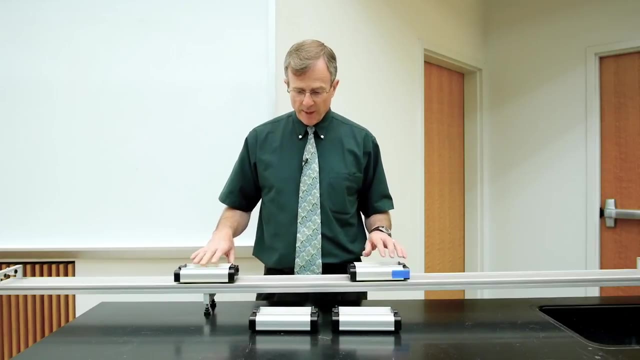 And when you solve the energy conservation equations and the momentum conservation equations, you find that all of the energy must be transferred from the one to the other. The other way you can do this is in the frame of reference of the center of mass of these two carts. 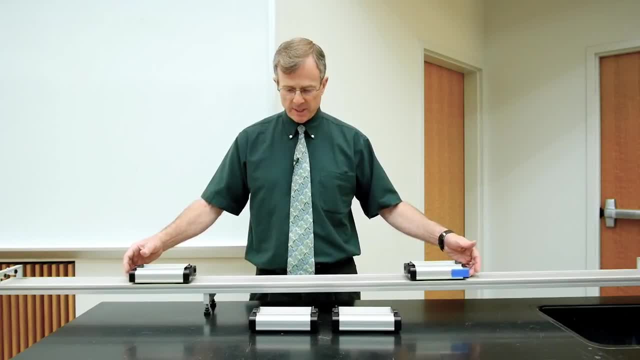 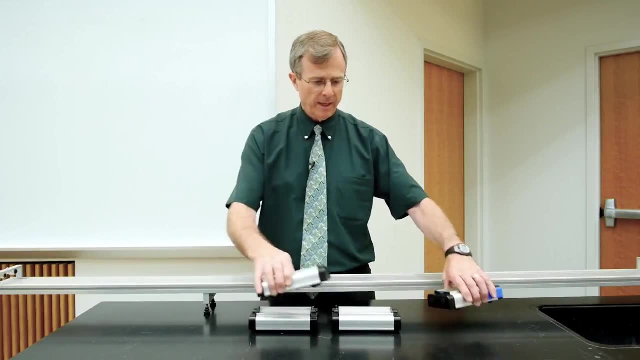 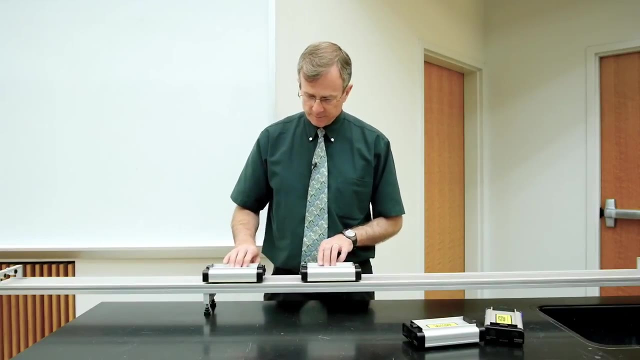 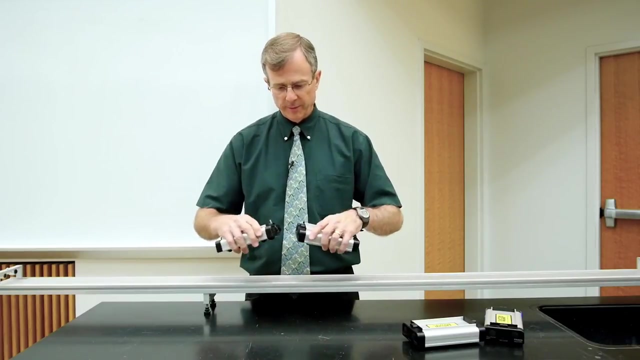 And if I'm capable of pushing them both at approximately the same speed, then they'll hit and leave each other at the same speed that they came together. These carts are different. They have no magnets, but they have some Velcro here and here on both of them. 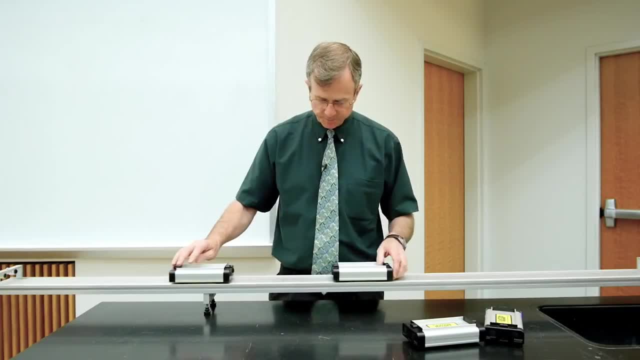 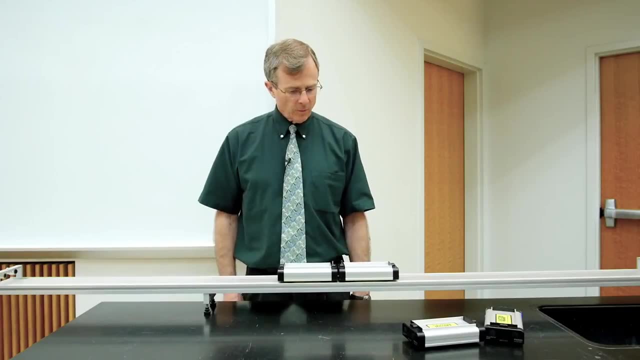 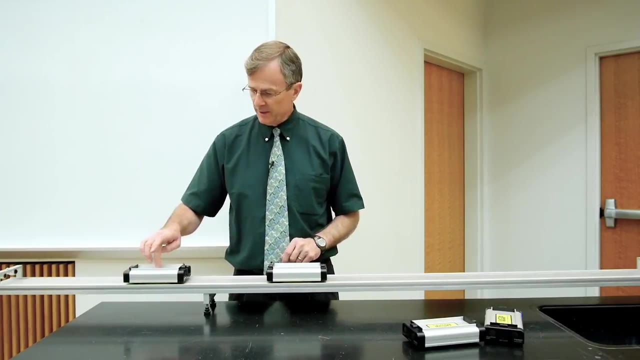 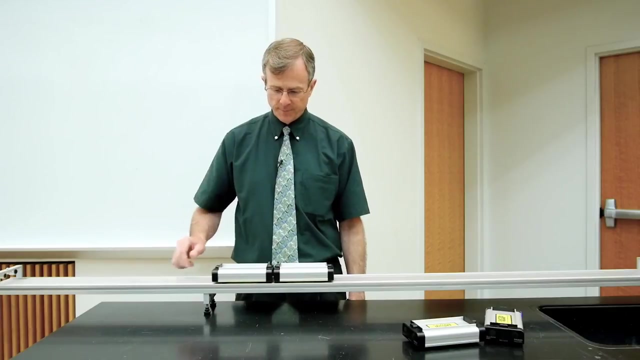 that allows them to stick together. So you start with this one stationary and this one moving. Then once they hit, then they move along together at a slower speed than this one was moving originally. This one has zero energy initially. This one has energy one-half mv squared. 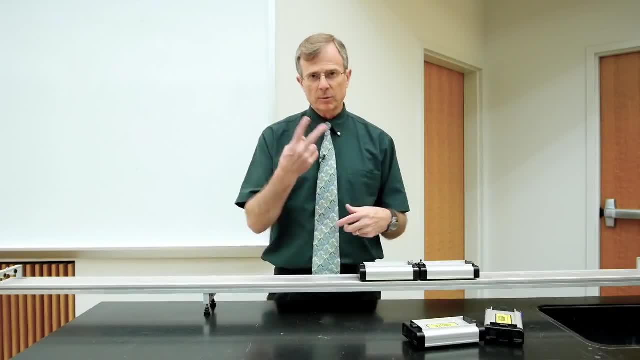 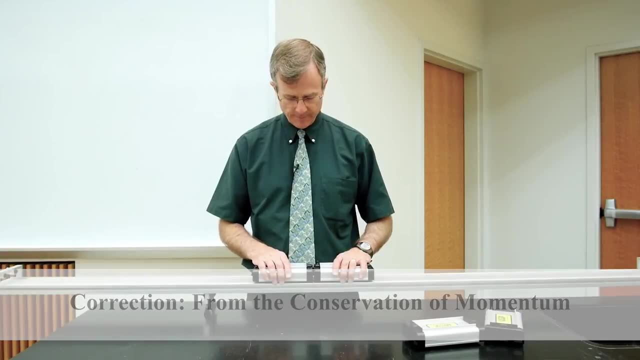 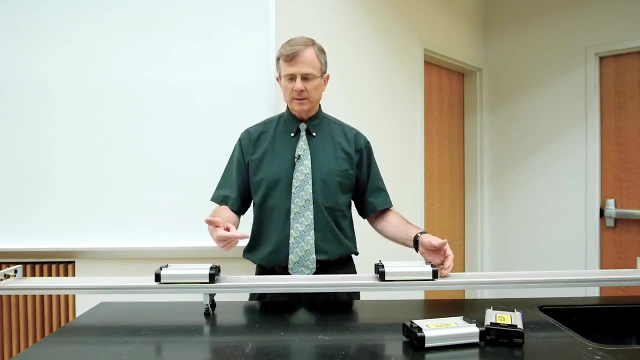 Once they hit, they move along as a unit with twice the mass and a smaller velocity that you can calculate from conservation of energy. You can also do this one in the center of mass frame, And if you impart the same momentum to this one, 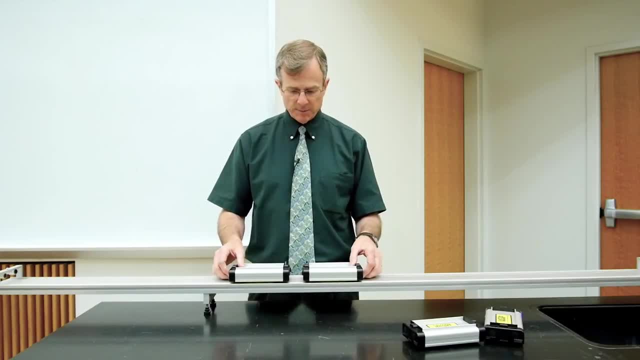 equal and opposite momenta to these two, then you can get them to stick and remain stationary just like that. That's a totally inelastic or perfectly inelastic collision.